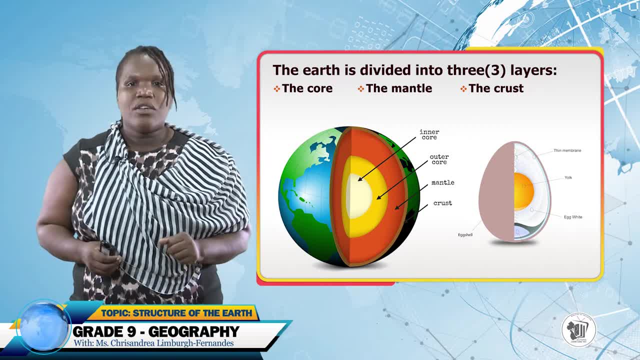 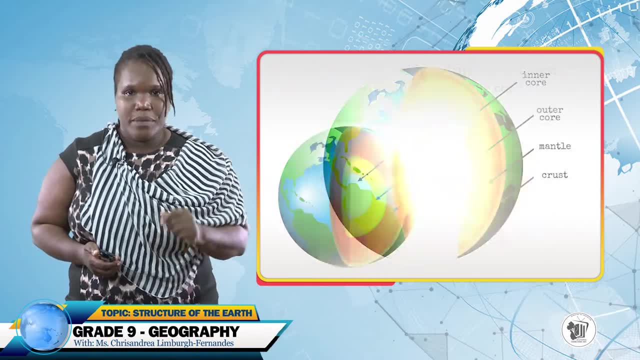 The albumen or the white part of the egg could represent the crust, The mantle could represent the mantle And, finally, the core could be represented by the yolk. Now we'll go into details about the parts or these layers of the Earth. 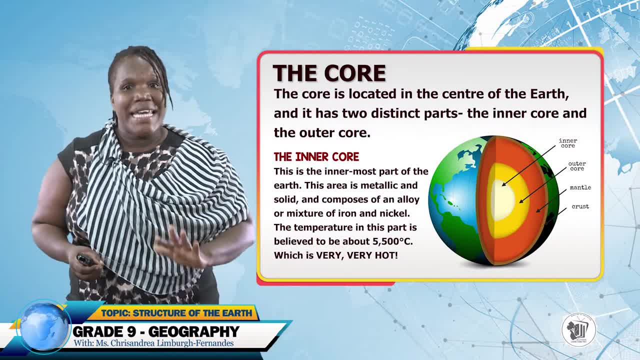 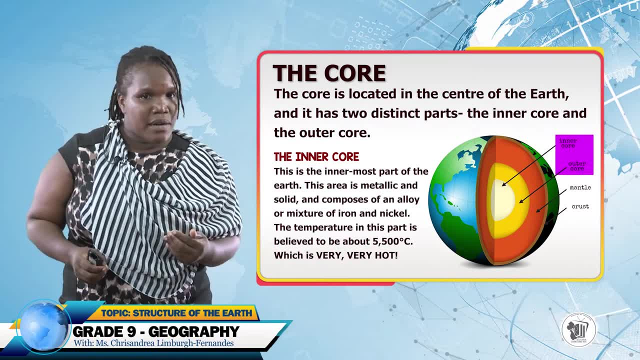 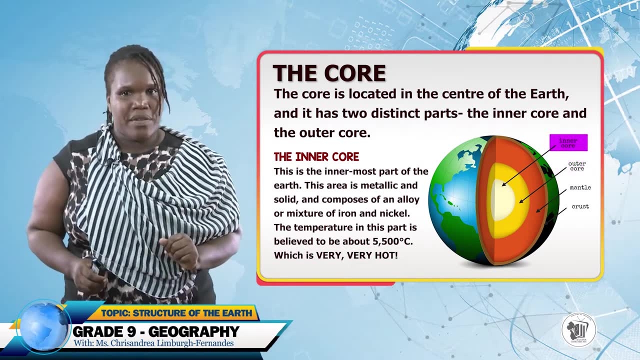 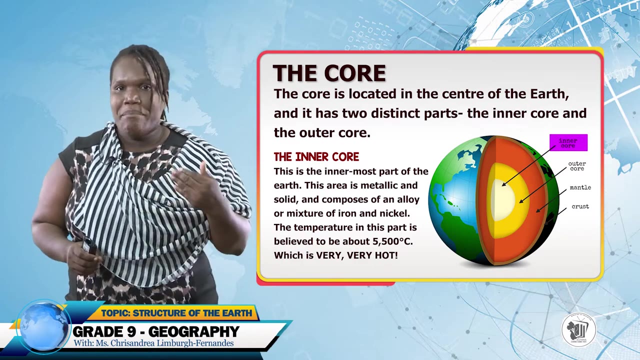 We'll start with the core Now. the core is located in the center of the Earth and it's divided into two distinct parts. These are the inner core and the outer core. The inner core is the innermost core. The inner core is the innermost part of the Earth and it is metallic and solid, and it's composed of an alloy or a mixture of iron and nickel. 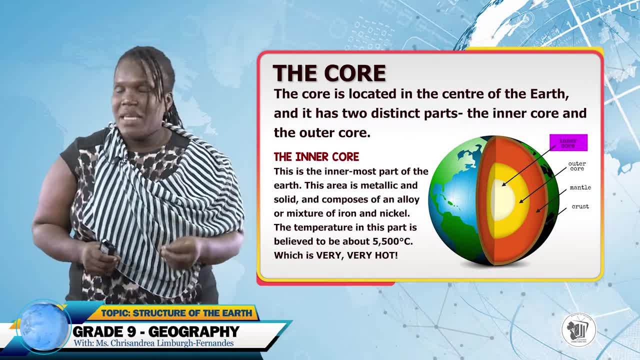 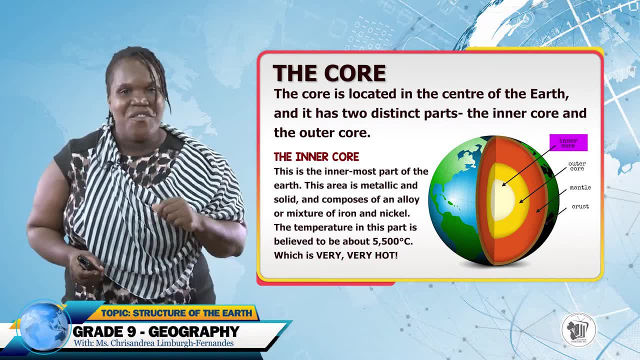 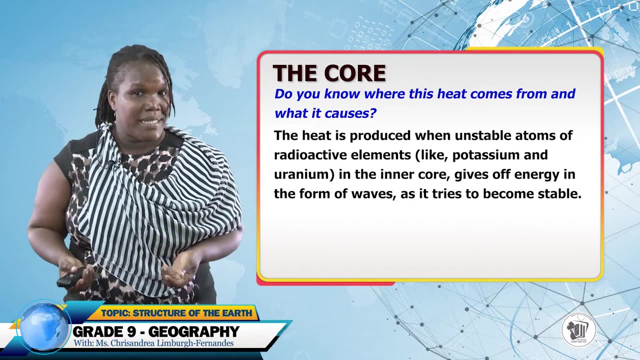 The temperature in this part of the Earth is believed to be about 5,500 degrees Celsius, And if you think of it, it's very, very, very hot. Now do you know where the heat comes from or what causes it? 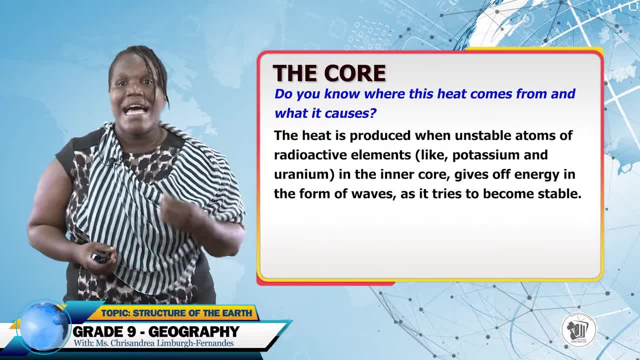 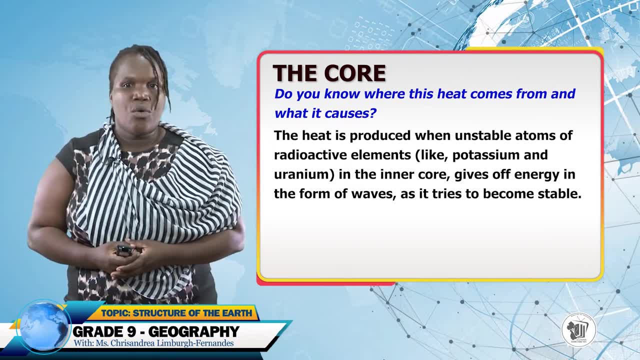 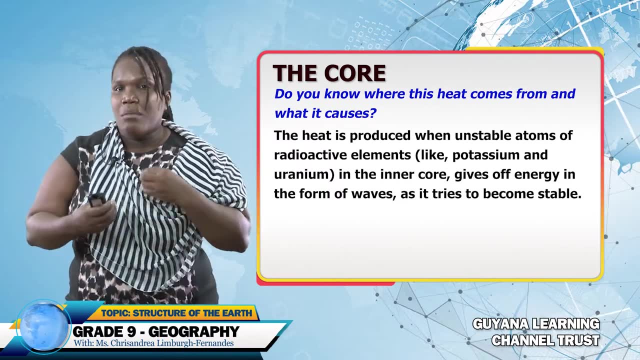 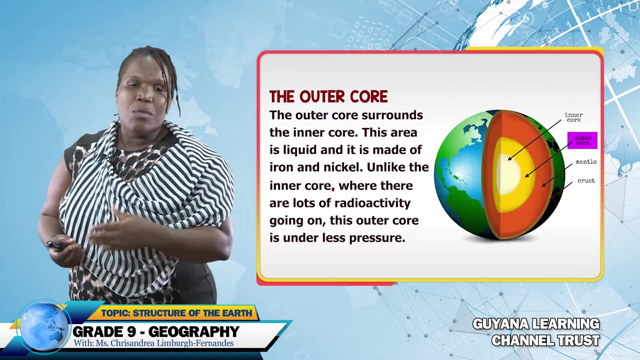 The heat is produced when unstable atoms of radioactive elements like potassium and uranium in the inner core gives off energy, And this is done as the atom seeks to become stable, right, And the energy is given off in the form of waves. Now what happens in the outer core? 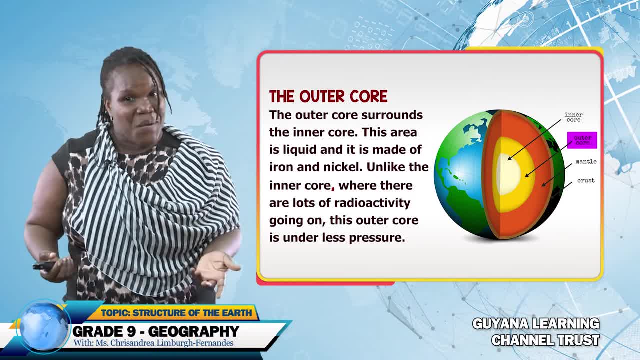 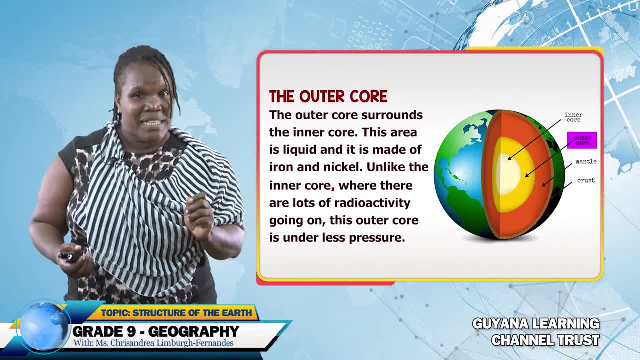 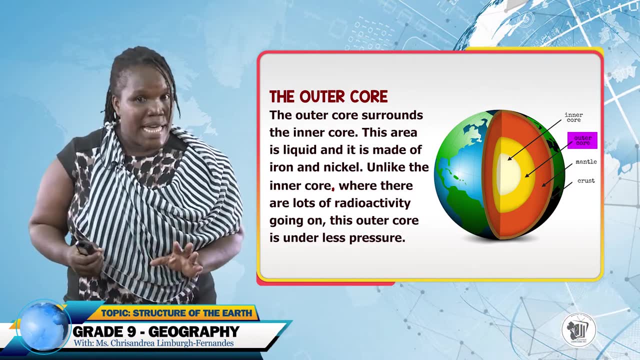 The outer core, as we know, surrounds the inner core. However, this layer is liquid in nature. It's also made up of nickel and iron, But, unlike the inner core, where there are lots of radioactivity going on all the time, this area is under less pressure. 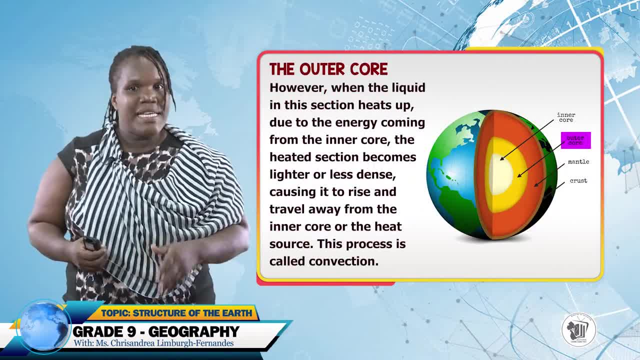 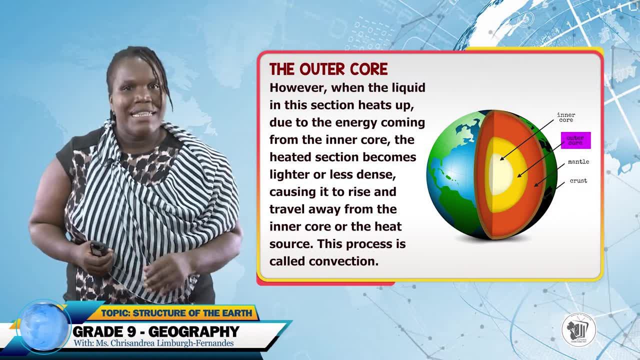 However, the liquid in this section heats up due to the energy coming from the inner core, and as it heats up, it becomes lighter, less dense, and this causes a lot of heat. And as it heats up, it becomes lighter, less dense, and this causes a lot of heat. 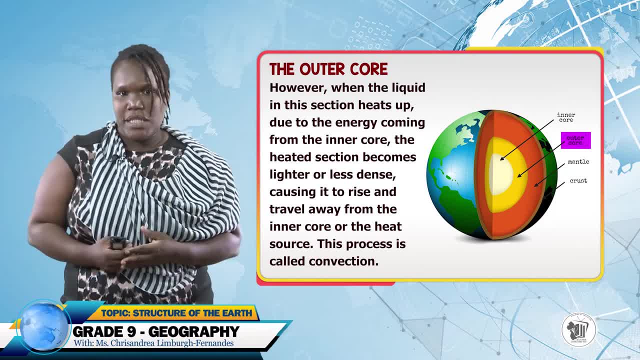 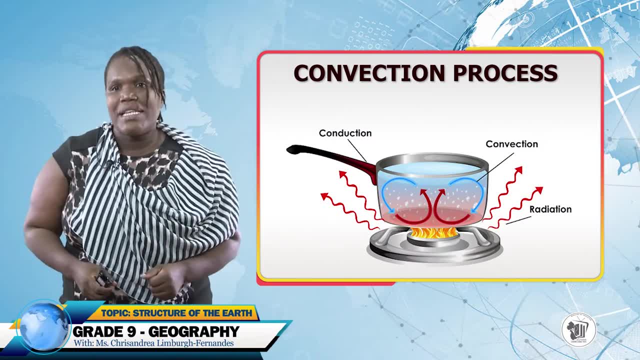 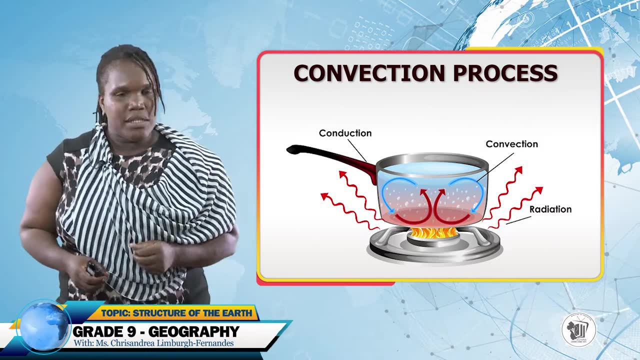 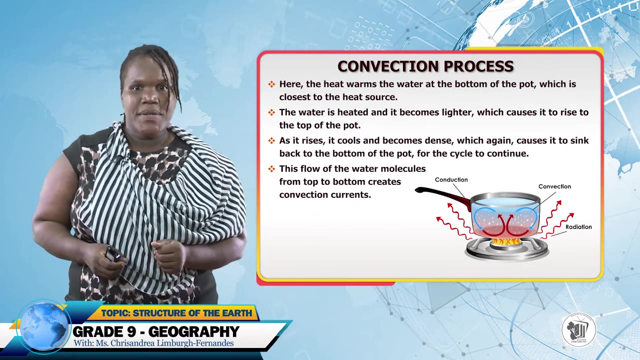 And this causes it to rise away from the heat source. This process is called convection. To understand convection and what really happens in the outer core, let's use the illustration of a pot of water on a stove. Here, the heat warms the water at the bottom of the pot, which is closest to the heat source. 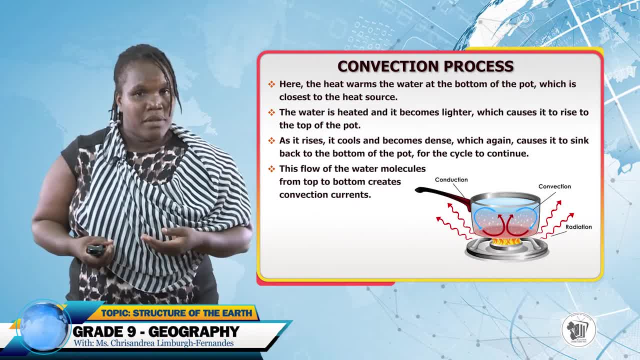 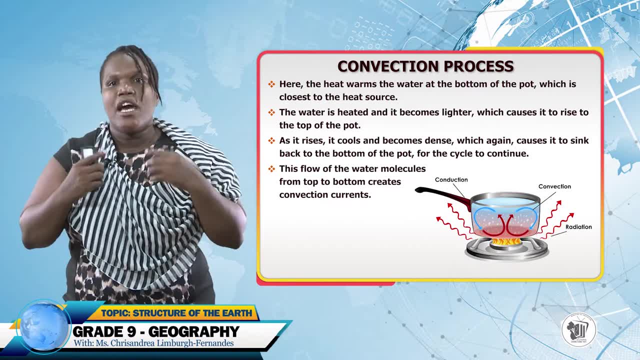 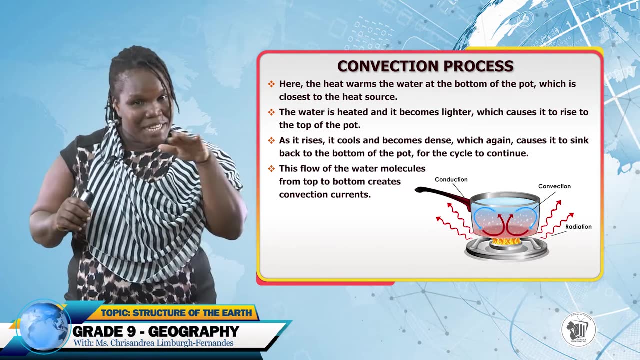 As the water molecules heat up, they become lighter And they rise to the top of the pot, And this is indicated by the red arrows. As the molecules rise, they cool, indicating the blue part of the illustration, the blue part of the pot. 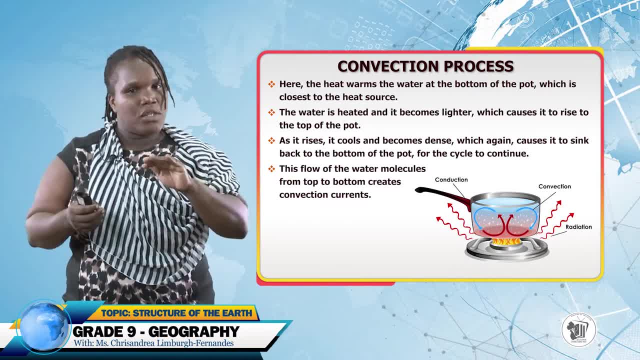 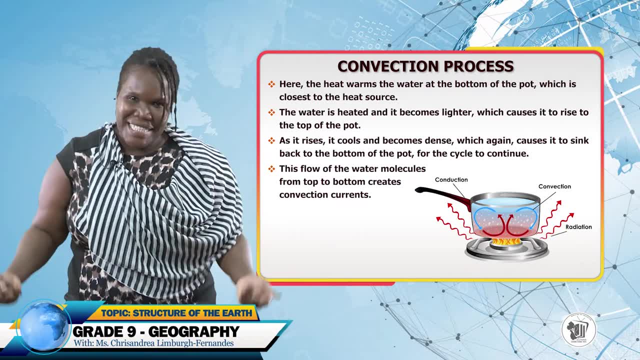 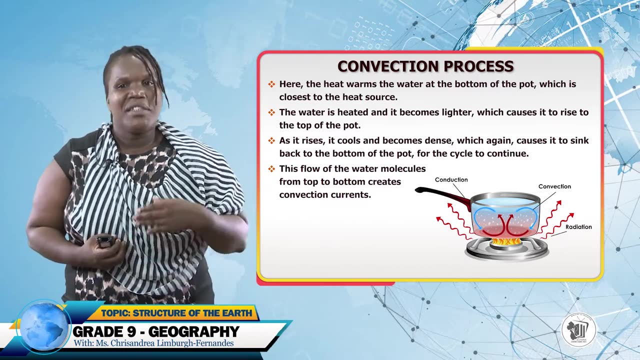 As the water molecule rises, it cools, And once it cools, it becomes heavy again. It's heavy so it sinks to the bottom of the pot. This cycle continues, And this is what is called convection currents. This is a fact you should note. 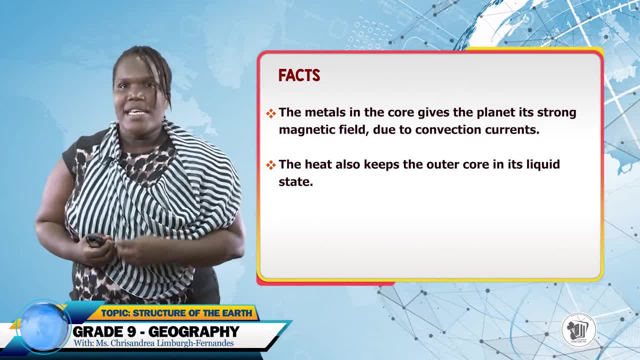 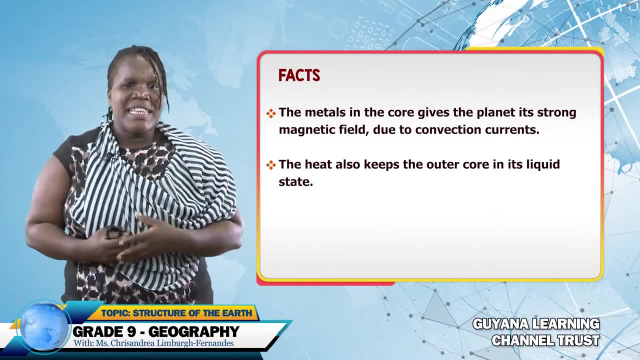 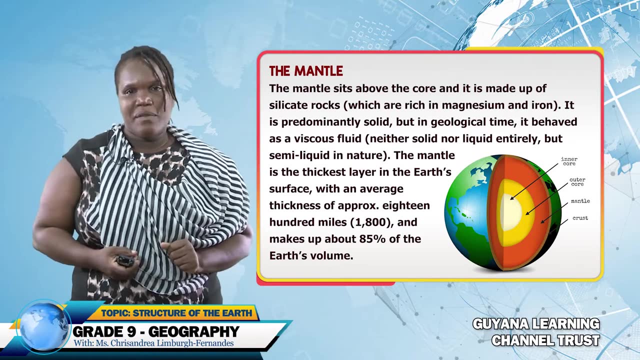 The metals in the core gives the planet its strong magnetic field And again it is due to the convection currents. The heat also keeps the outer core in its liquid state. Now let's talk about the mantle. The mantle sits above the core. 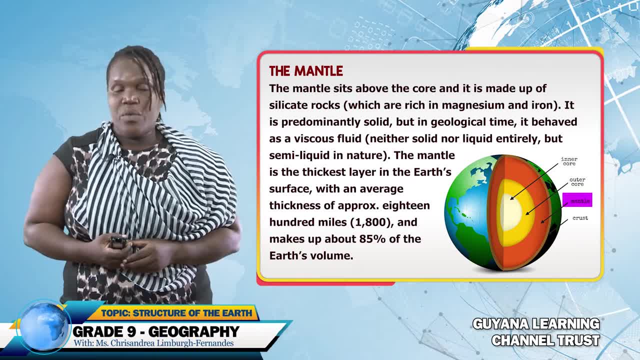 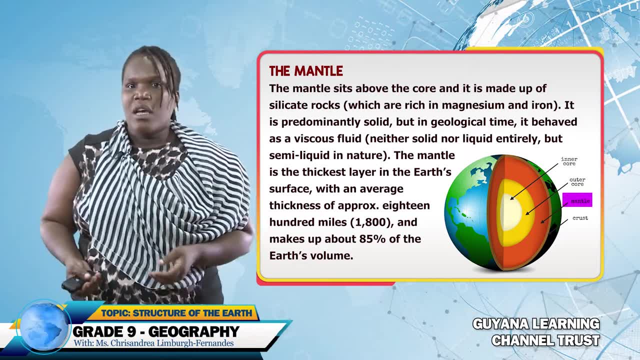 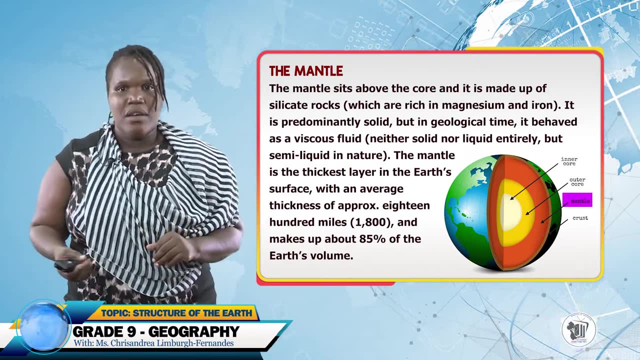 And it is made up of silicon, Made up of silicate rocks Which are rich in iron and magnesium. This area is predominantly solid. However, in geological time it behaved as a viscous fluid, Being neither solid nor liquid, But in a semi-liquid state. 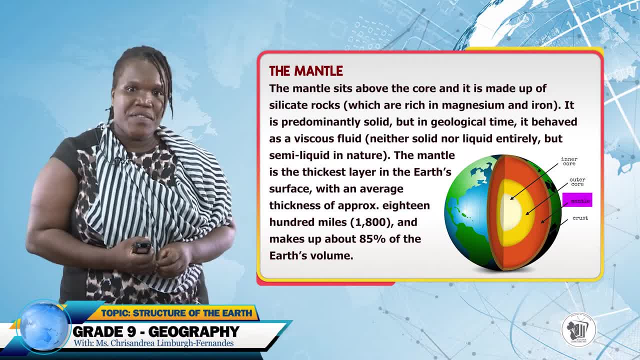 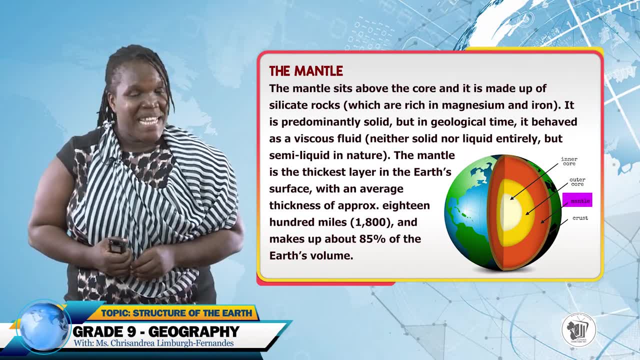 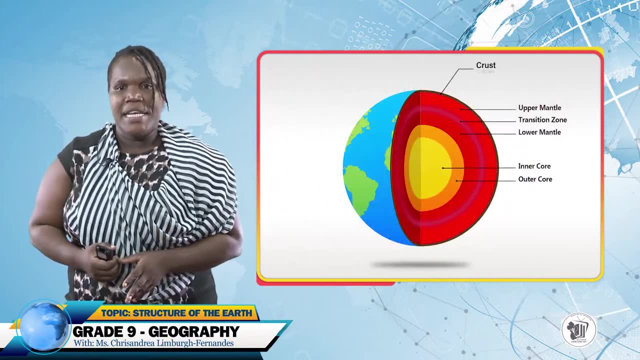 You should know that the mantle is the thickest layer on the Earth's surface, With an average thickness of approximately 1800 miles, Wow, And it makes up about 85% of the Earth's volume. Note that this layer is divided into several components. 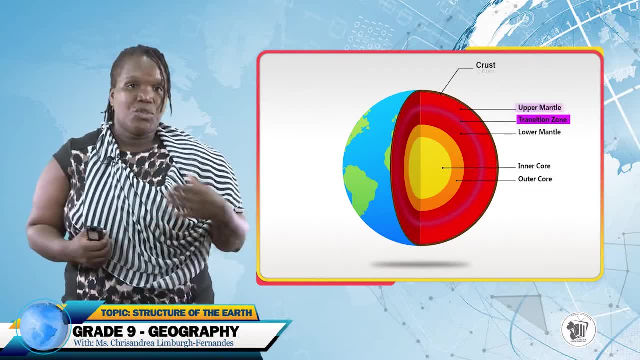 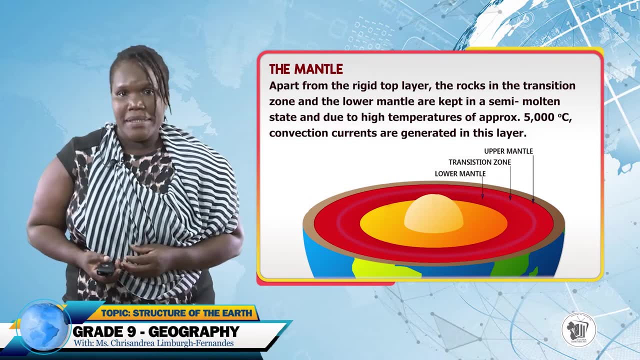 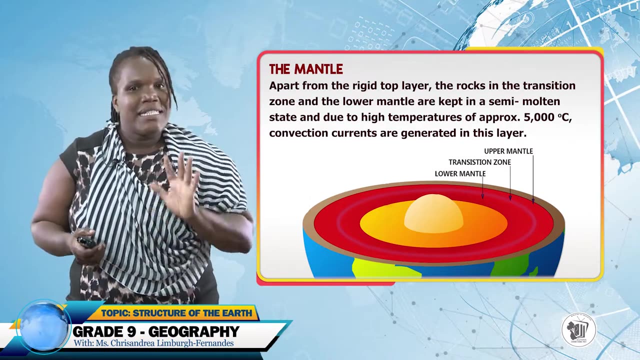 Three of which are the upper mantle, The transition zone And the lower mantle. As part of the rigid top layer of the mantle, The rocks in the transition zone and the lower mantle, They're always kept in a semi-molten state. 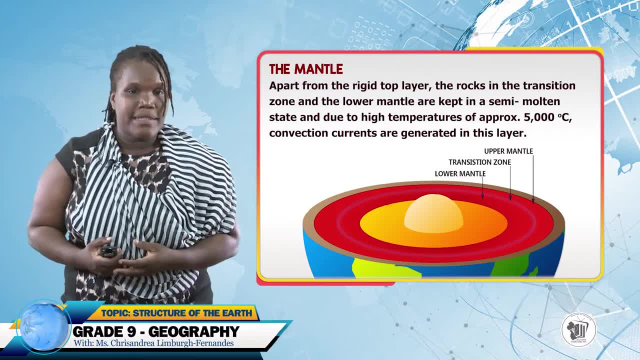 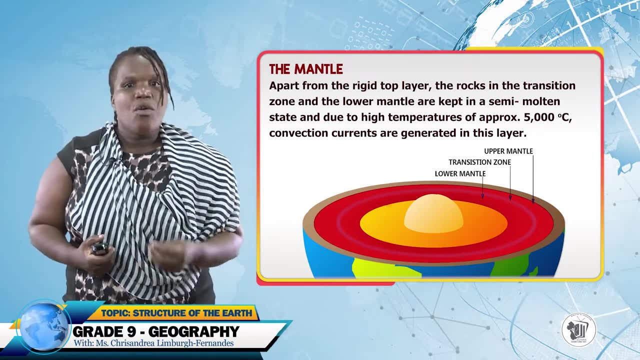 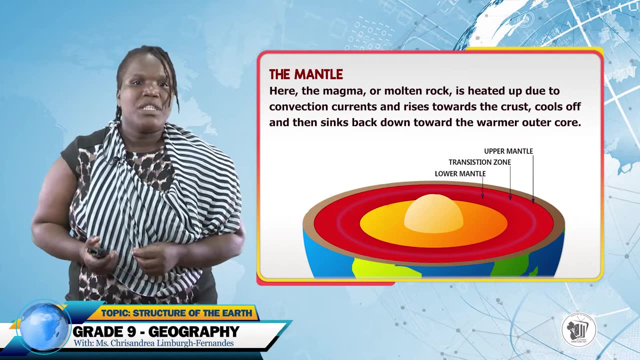 And this is due to the high temperature that exists there- Approximately 5000 degrees Celsius- And convection currents are also generated in this layer. Here the magma, or molten rock, is heated up due to convection currents. Again it rises to the top of the crust. 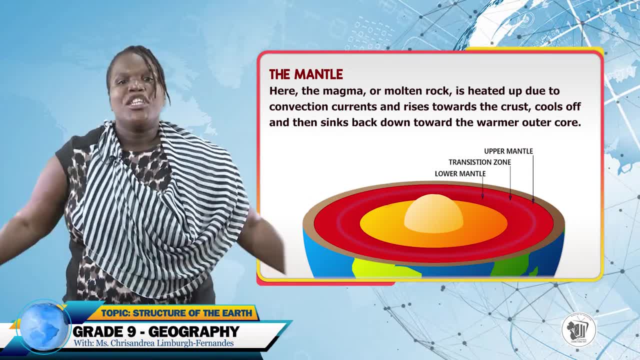 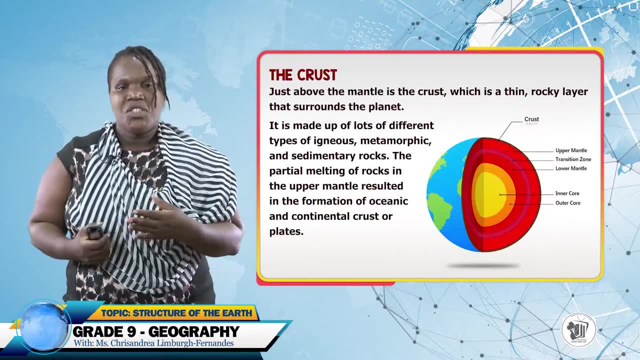 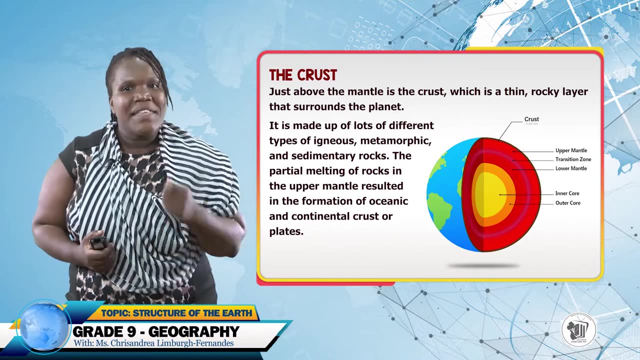 Cools off And then sinks back to the bottom of the core, Where it's much warmer. We'll now talk about the crust. Just above the mantle lies what we call the Earth's crust. This is the thinnest layer. It is also rocky. 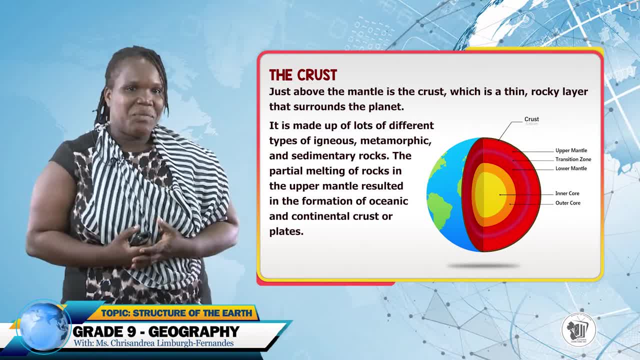 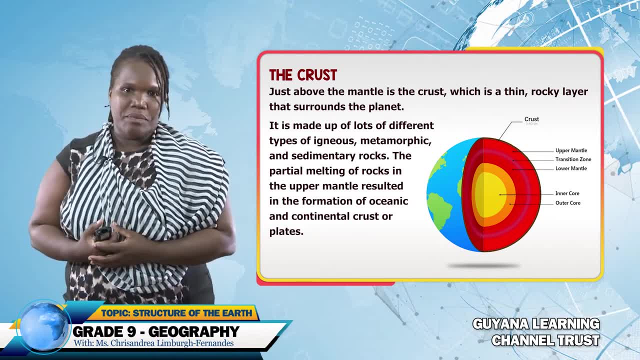 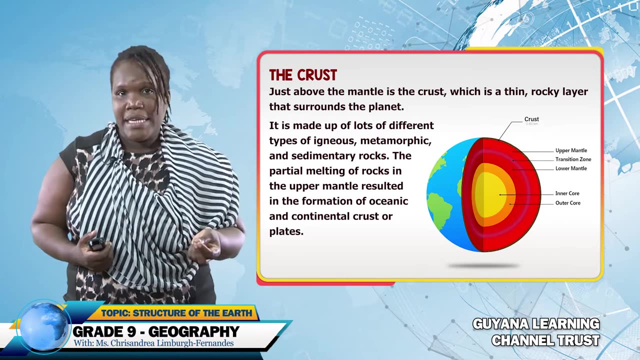 And it surrounds our entire planet. It is made up of all different types of igneous, metamorphic and sedimentary rocks. The partial melting of rocks in the upper mantle results in the formation of what is called oceanic and continental crusts, or plates. 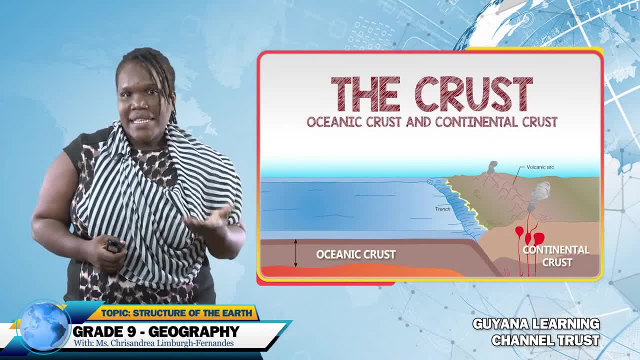 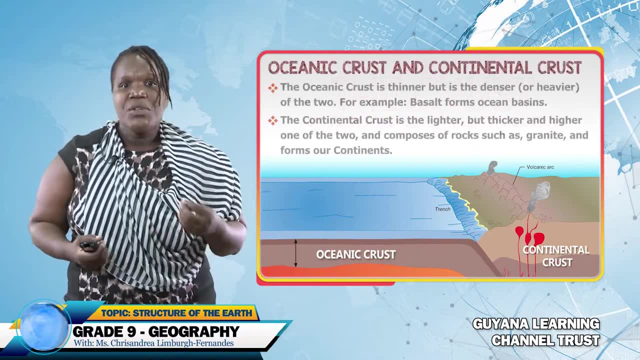 Here's a brief discussion on what is the oceanic crust, What it's made up of, What is the continental crust And what it's made up of. The oceanic crust is the thinnest but denser of the two crusts. 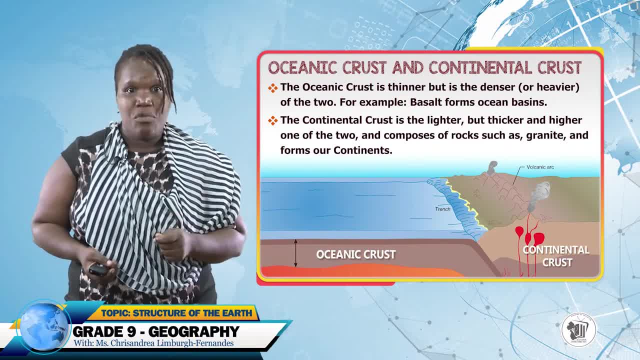 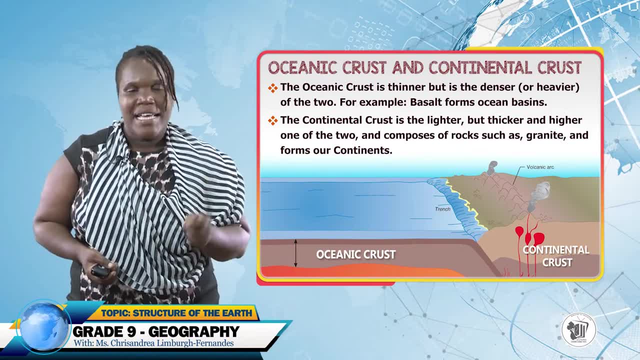 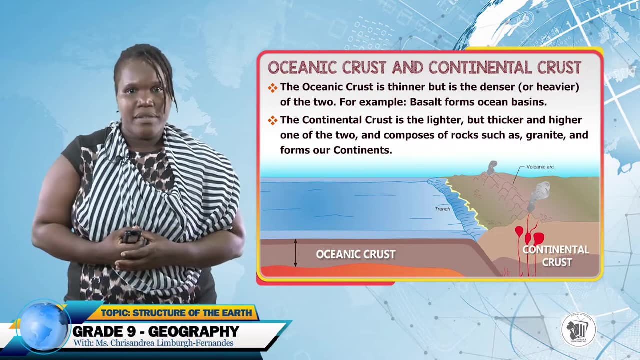 Right. It is made up of basalt rocks And they form the ocean basin. I want you to remember, Oceanic crust is thinner and denser Right, While the lighter of the two is the continental crust. This crust is also thicker and higher. 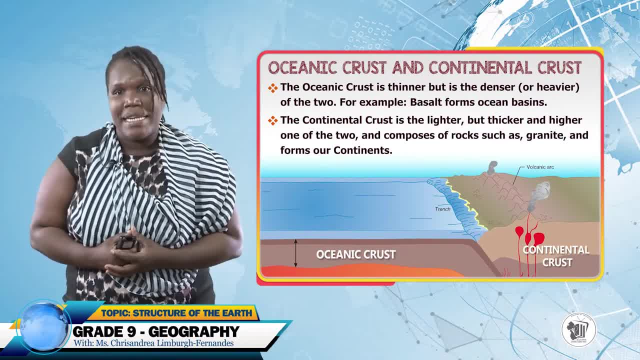 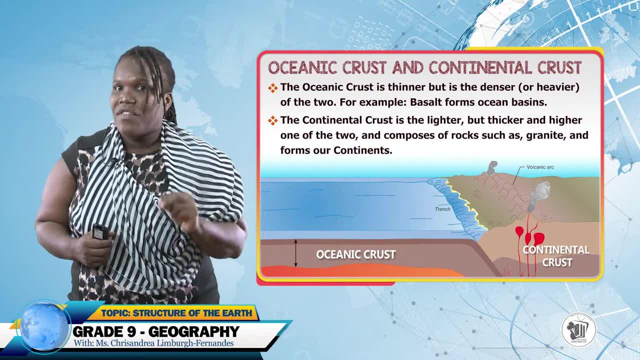 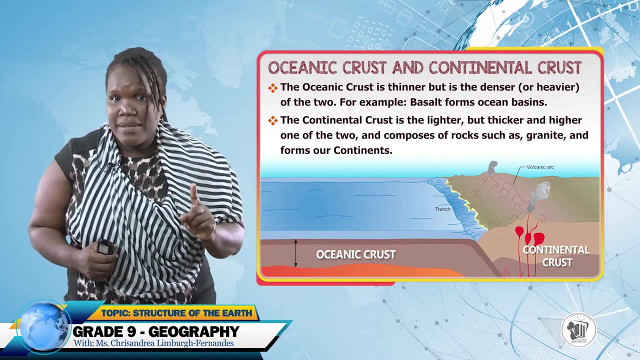 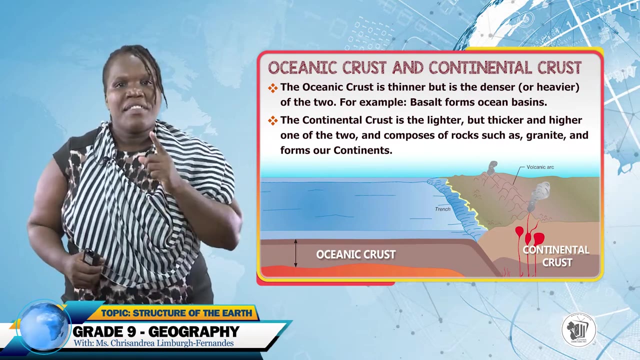 And it composes of rocks such as granite, And they form our continents. You must remember this, students. These two facts are critical facts That will carry us through our geography. Oceanic crust is thinner and denser. Continental crusts are higher, thicker and lighter. 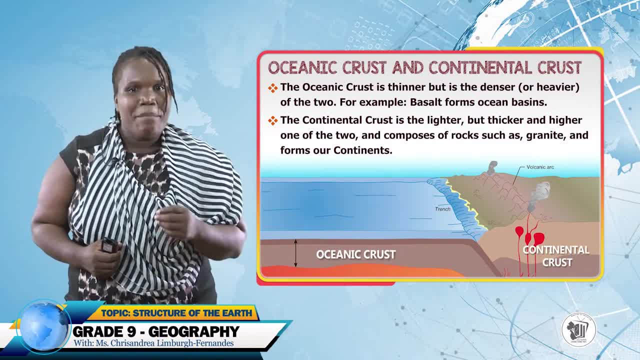 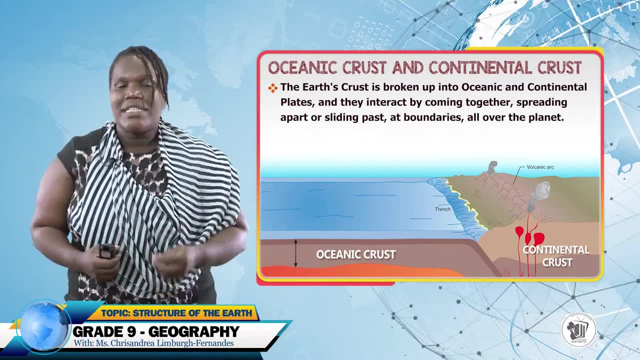 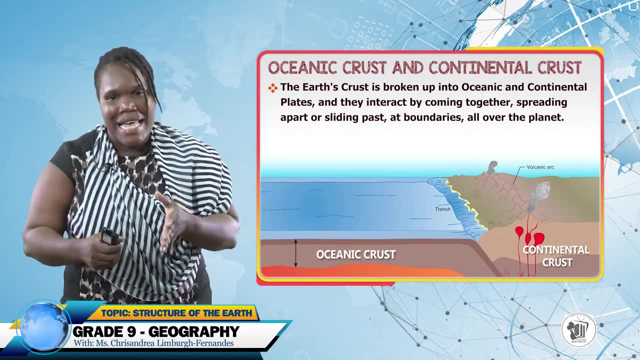 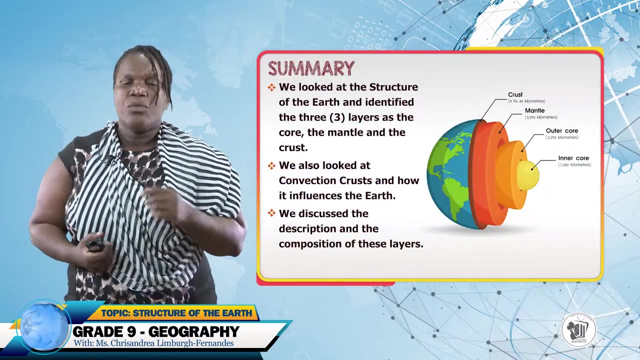 Finally, for emphasis, Remember that the earth's crust is broken up into oceanic and continental plates, And note that they are always in interaction, Coming together, spreading apart or sliding past one another All over our planet. In summary, We looked at the structure of the earth.